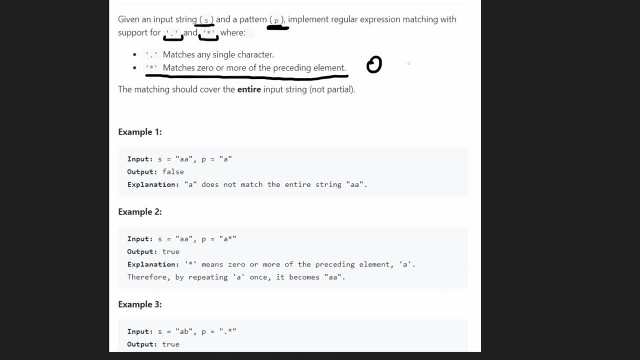 right, so it can be repeated as many times as it needs to be. and the match or the pattern has to cover the entire input string, so it has to match the full input string. So one example is: let's say so these are the special characters we worry about: right, the period and the star. if we don't have 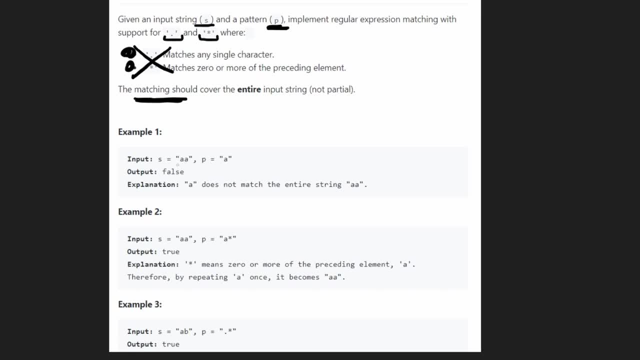 either of them, then it's basically string matching, right. so we see in this example we have two a's, right, that's one input string and a single a. so basically, do these strings match each other? they don't match each other, so we have to return false meaning. 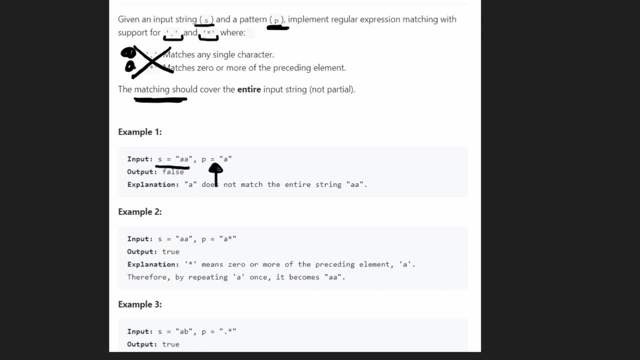 that the input string s does not match this regular expression- and, remember, it's only going to be a regular expression- which possibly has the star or possibly has the period. Now imagine instead if our pattern was a period. so in that case we would compare it to the string double a and we would see that, yes, they do match because, remember, the period can. 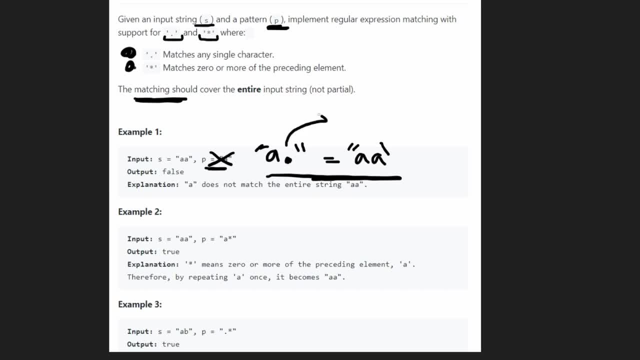 be any character, so we could say: okay, well, given this pattern, this could be double a, so it would match this input string. what if we were checking: does it match this input string a- b? in that case it would also match, because this period could then turn into a- b, so it would be a, b and these: 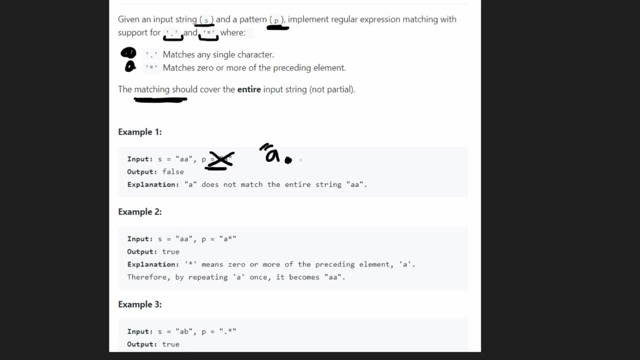 two match each other. but of course, if we had a period period checking if it matches double a, it doesn't, because they're not even the same length. this has three, this has two. there's no way we could put any characters for these two periods that would match. 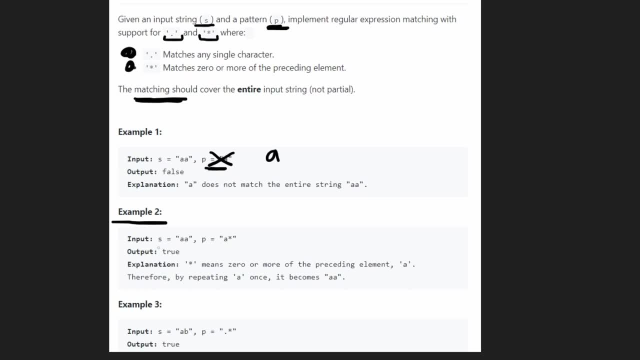 double a. and what about this second example? let's say the input string is double a and the pattern is a star. so what this star means is a star. so a star basically means that the element that comes before this a could be repeated multiple times or zero times. 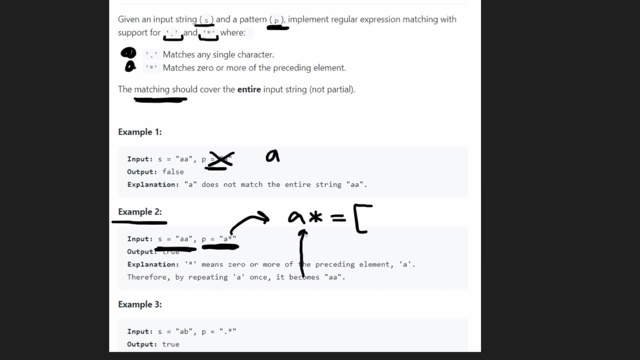 so the possible strings that this pattern could match to could be an empty string, because this character could be repeated zero times, right, so empty string. this character could be repeated once, so a single a. this character could be repeated twice, so double a. this character could be repeated three times, so triple a, and so on and so on. right, we could repeat this, a infinite number. 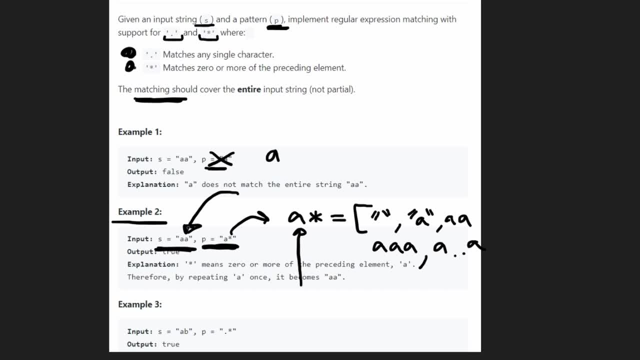 of times. but if you take a look at our input string, we're only checking: does it match double a? of course it does, right, we just repeat the a twice. so in this case we return true. a third example: so let's say our input string is a- b and we're checking: does it match the pattern dot star? 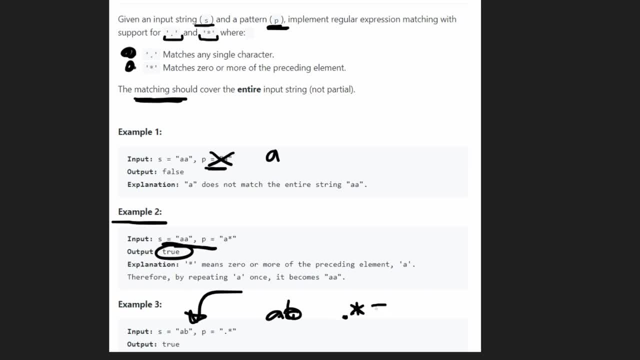 so basically what this dot star means is we could have a string that's empty, right, repeating the dot zero times, so empty string. uh, we could repeat the dot once, so dot. we could repeat it twice, double dot, right, and so on and so on. and so let's say this: right, double dot is what we're looking for. we're checking: does this match a, b? 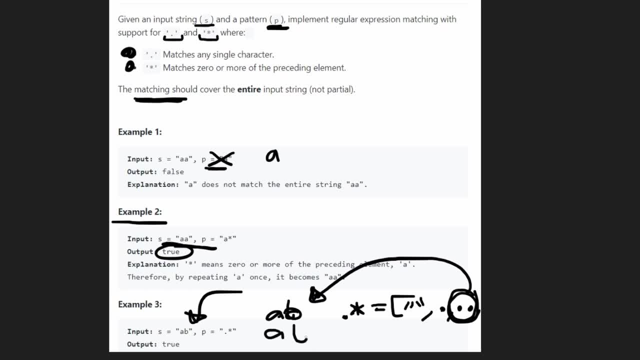 well, one of the dots could be a and one of the dots could be b, so that matches double dot. so this would return true. so, as you can see that there's probably going to be a few edge cases we have to deal with, right, the complexity really mainly comes from the star, the dot isn't so. 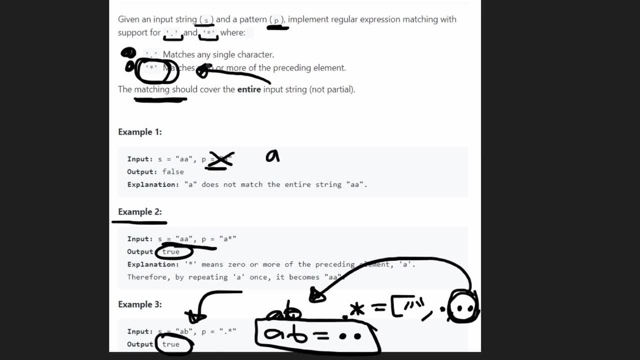 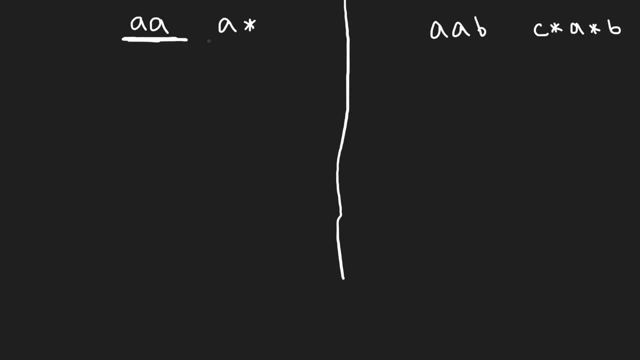 difficult, right, but the star makes things interesting. so let's just try to brute force this. so let's just look at one example. this example: let's say: this is our string s and this is our pattern: a star. so, as you know, the star is really where the complexity comes from. so let's make a 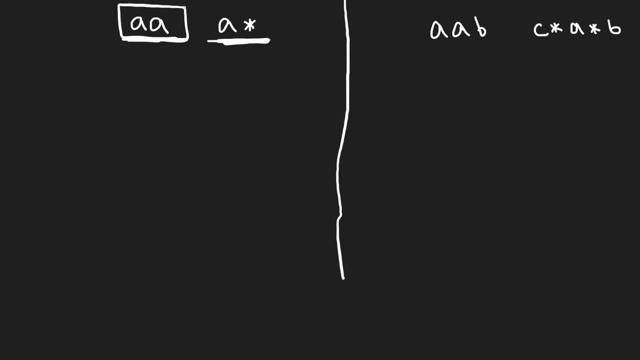 decision tree. let's brute force this. so this is the string we're trying to match to. this is our pattern: a star, we know. so we're first going to look at the first a and then we're going to look at the first character of this. now, this isn't just an ordinary character, there's a star that can be. 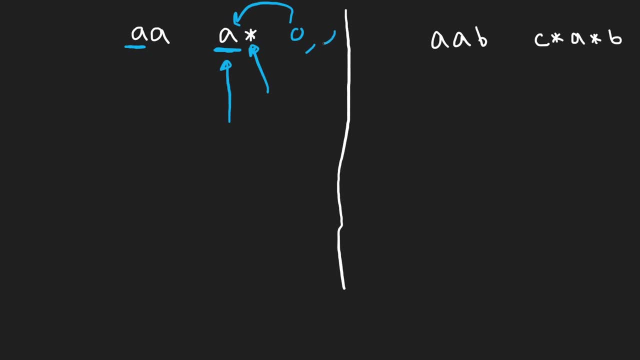 repeated with the second letter a, so this could be repeated minus a or for whatever reason. number b plus a, zero and minus b plus c plus a and a half next to each other, right? so once this background comes after it. so this could be repeated zero times or more times, right? 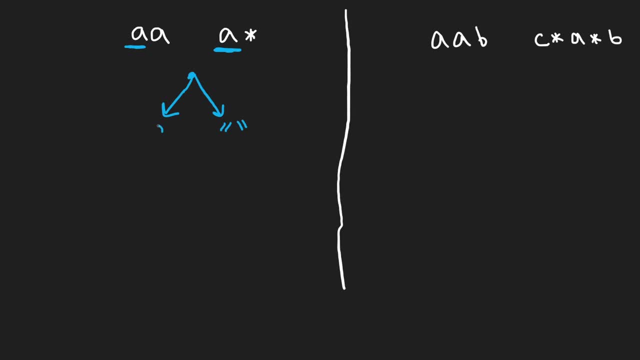 so let's brute force this. we know we have a choice. are we going to repeat the a at least once, or are we going to repeat it zero times? if we repeat it zero times, then we end up with an empty string. right. if we repeat it once, we end up with a single a. now, clearly we want the single a. 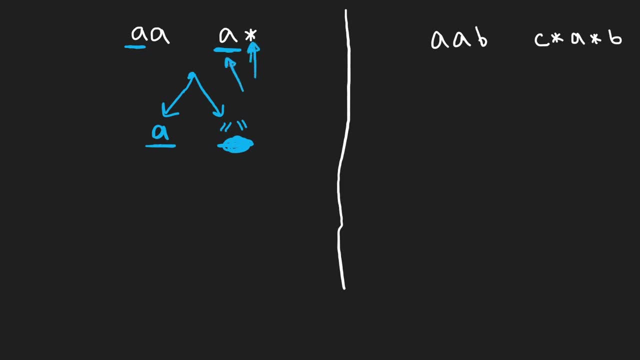 empty string, meaning we want this star to or and this character a to repeat zero times, then we would have to move to this position, right, and there clearly isn't any character here. maybe there would be a b, maybe there would be an a, but there's clearly nothing there. so this is, this decision is. 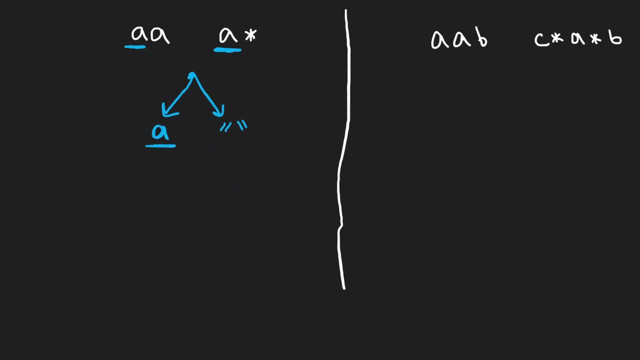 going to stop right. we cannot go any farther. all we can do here is an empty string, but it's okay, because we ended up matching with this a when we were on this path, right. so now the character we're looking to match in the input string is this single a. so now, again, we have a choice, are we? 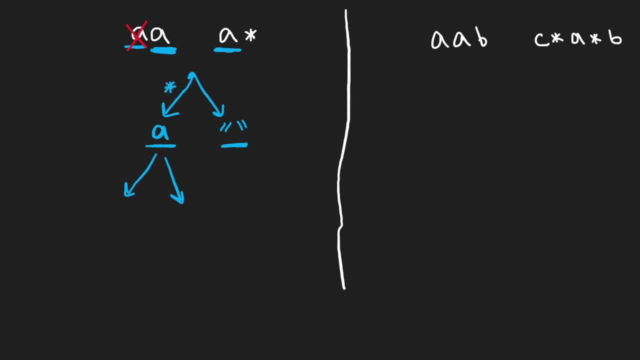 going to repeat the star, like in this spot. we repeated the star. in this we didn't repeat the star. now again, we have that choice. are we going to repeat the star or are we not going to repeat the star? if we don't repeat the star, we're going to end up with a single a and then we're going to 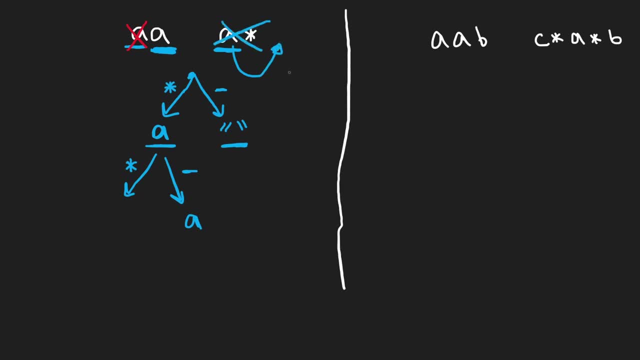 have to be sure, the input string was a double a. so really our other decision, where we do repeat the star at least one more time, is going to lead us to double a. and that's good, because now we have the second a, meaning we matched this second a right. so now in reality we have matched the input string. but 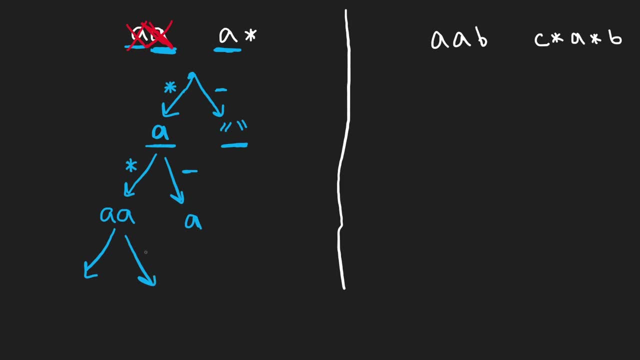 just to show you. in the next step, we're going to have to repeat the star again. so we're going to, in theory, we could keep going. we could decide not to use the star anymore. right, we would be shifted to that position, and in which case our ending string would just be double a. 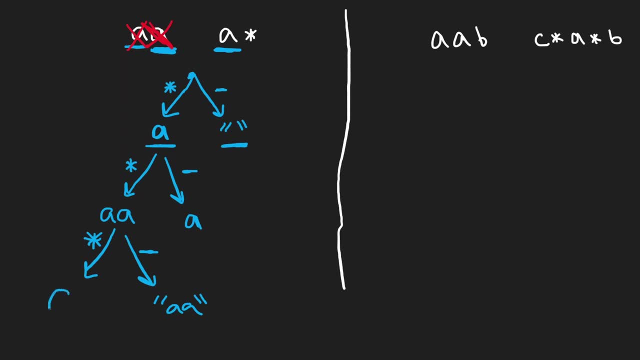 or we could use the star one more time, meaning we'd get triple a, but then of course you can see we're even bigger than the input string that we wanted to match. so we stop. but we see that we did end up finding the result. since we found the result right, we found the input string. that means: 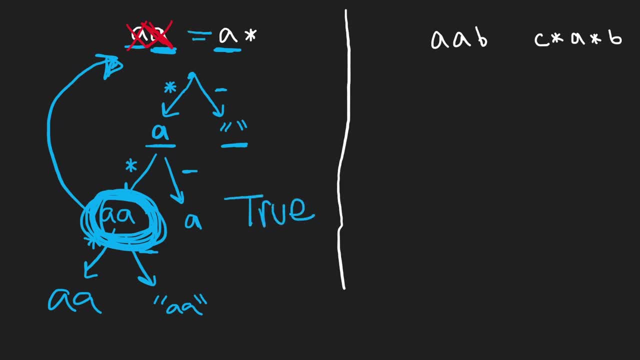 that these do match right. so we would return true because the input string matches the regular expression. but, as you can see, we're doing a decision tree. this is not exactly going to be super efficient, right? how many decisions are we going to have? well, anytime we get to a star, we're. 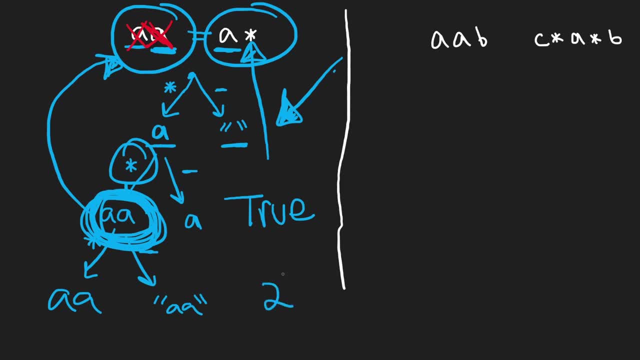 going to have two different decisions. how many times can we repeat that decision? it's going to be n, where n is the input string s. so clearly you can tell this is not super efficient. but in case you haven't noticed, this is a dynamic programming problem and if we take this and we implement a 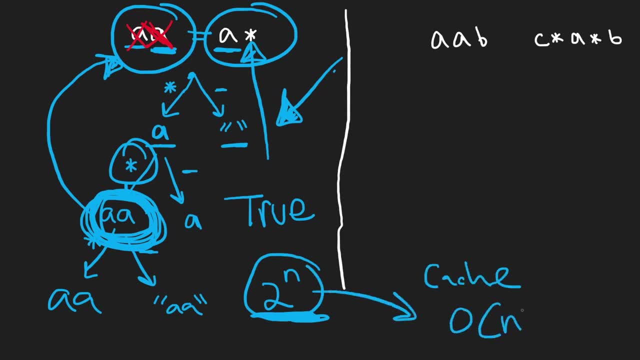 cache, then we can get this time complexity down to n squared, or in other words, really we're getting it down to n times m, where n is the length of the input string and m is the length of the pattern. and this is if we do the top down memoization with a cache we can also do the actual bottom. 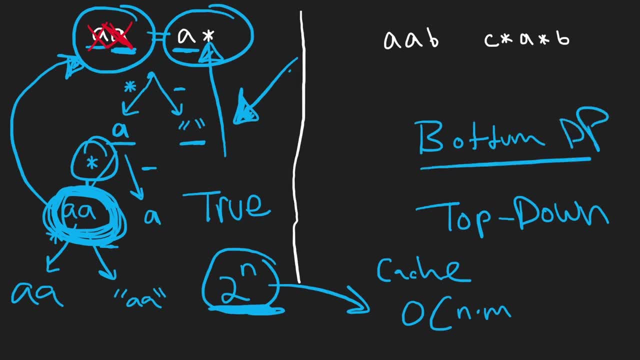 up dynamic programming solution, so the bottom up dynamic programming solution, and both of these actually have the same time time complexity. so i'm going to show you the top down coding solution. but once you know the top down solution, getting the bottom up full dynamic program solution is. 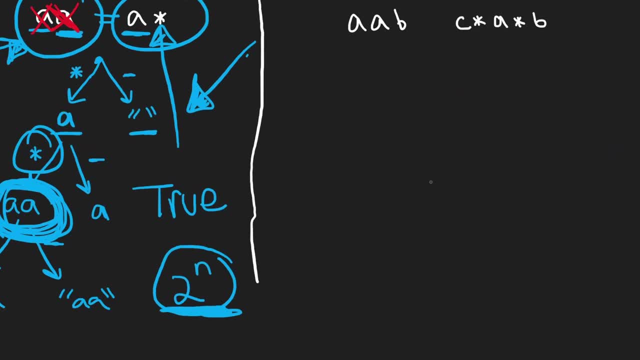 not usually impossible. but before that let's look at one more example. so the index i'm going to use. so let's say this is our input string s and this is our pattern p. so i'm going to use two variables to keep track of where we are in each of. 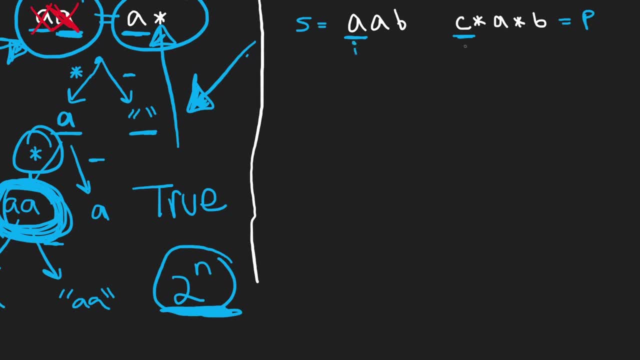 the strings. i'm going to use i to tell us where we're at in the input string. i'm going to use j to tell us where we're at in the pattern. so remember, whenever we reach a character that has a star that comes after it. we have two choices. so i'm going to draw our decision tree we have 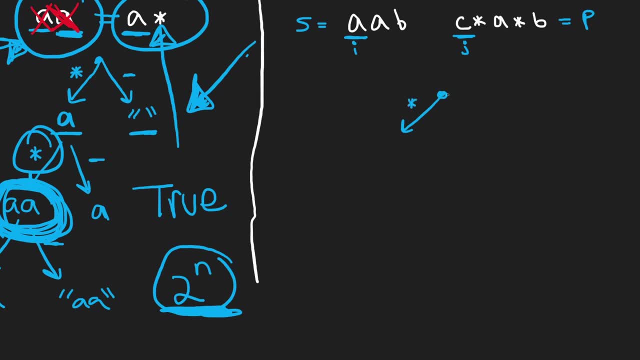 a choice to use the star, or we have a choice to not use the star. so in this case, if we use the star, use the star meaning we use the character at least once- we're going to get a C right. We're going to repeat the C just once. If we don't do that, we're going to get an empty string. So I'll. 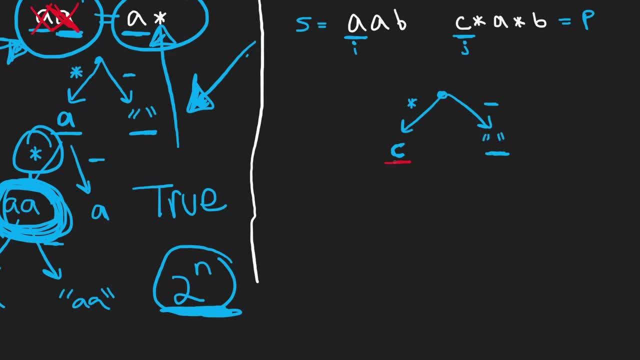 just draw this dash for empty string. Now you can see we have a C, but the first character of our input string is A. So really, what we want to do is not use this C any times, meaning we do not want to use the star, We don't want to repeat C even a single time. So the decision we want is not: 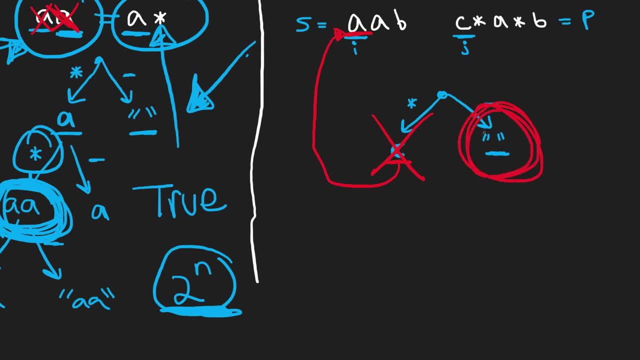 this decision, but this is the path that's going to lead us to the correct answer. So what am I going to do with this J pointer? I'm going to shift J. So I'm going to shift J over here, right, So? 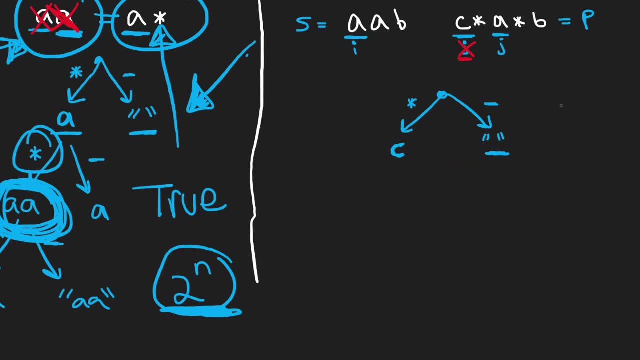 notice what we just did in this path where we do not use the star. right, We didn't use the star. What did we do? We ended up shifting J by two, So we took J and then added two to it. That's very important. 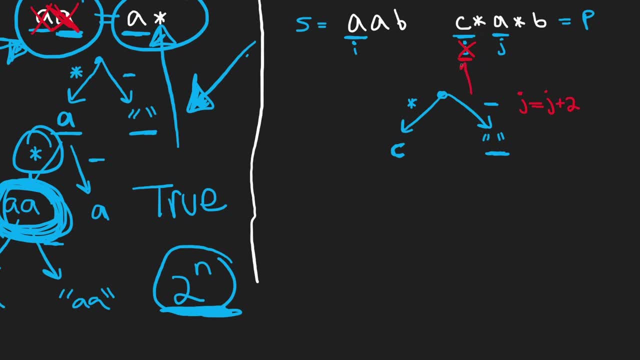 because any time we choose not to use the star, we're going to take our pointer where it's at and then shift it twice, because we're shifting one to get to the next character, But also look at the star. We don't want to land on the star, We want to land at the next character. And what about? 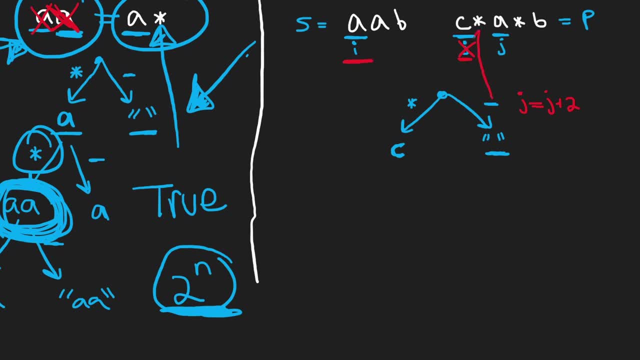 pointer I. Are we going to shift that? Well, since we didn't use the star, that means we weren't able to match with the character A Right. So actually, I is going to stay exactly where it is. So in this decision, what we did is: 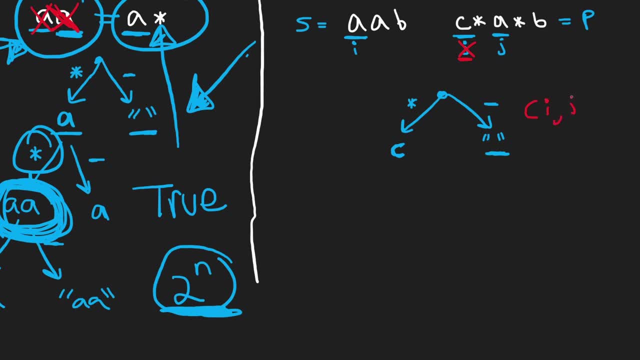 we left I the exact same, and then we took J and added two to it, And this is very important because this is exactly what I'm going to do in the code. So I remains the same: J plus two. Okay, so now we're still at this A, but our J is over here. So notice how J right after J is a star. That means 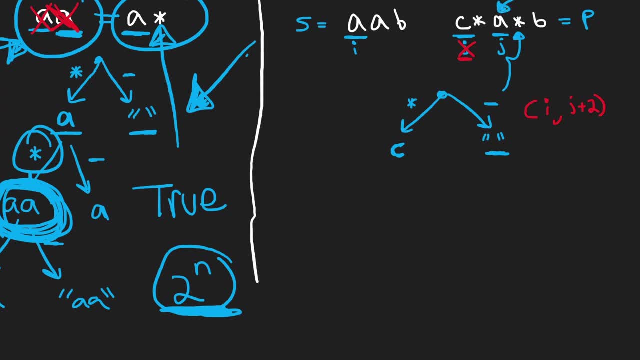 we can. we can be repeated zero times, or it can be repeated one or more times. So again, we have a decision to make. So one decision is: we use the star at least once. The other decision is: we do not use the star at all. So if we use the star once, we'll get a string of A. If we don't use 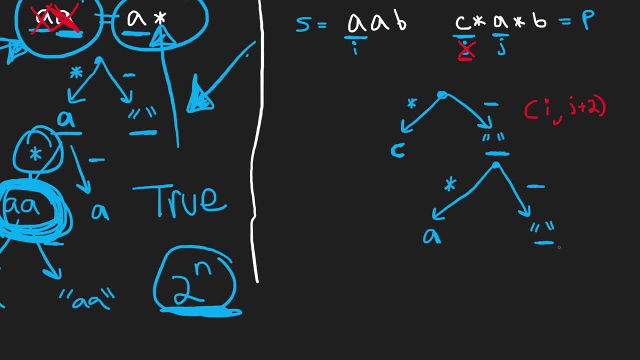 the star again, we'll end up with an empty list or an empty string. So remember, when we use the star over here, we got to see that didn't match the A, But now we actually have an A that isn't exactly matches the character over here, right, But what about this path? right, Right now we have 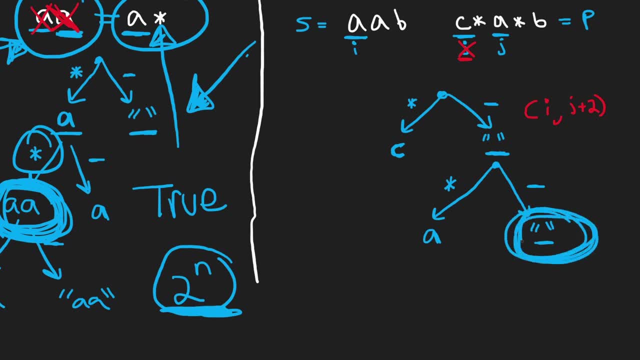 an empty string. Is this path going to lead us to the correct answer? Well, the only way to find out would be to continue on this decision tree, right making decisions and stuff. But I'm not going to show that because it's going to get pretty messy And you can tell by looking at the string, since 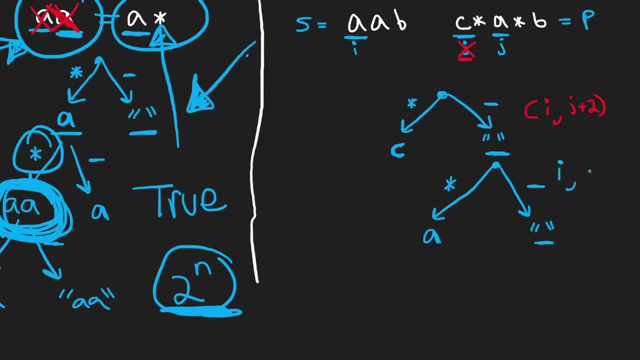 we chose this path, we would have to leave I as it is and we'd have to add two to J, So I would stay with the I as it is. And then you see, the pattern left at this point is just B. Does that match the? 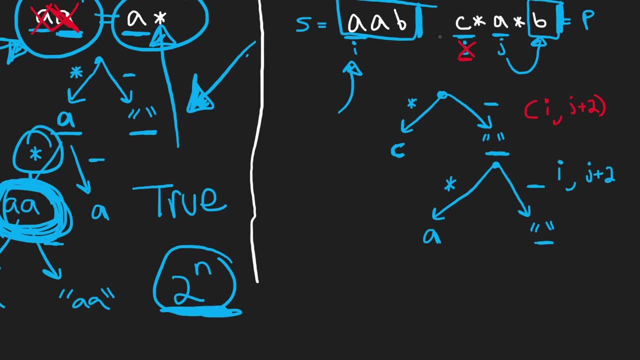 input string S. It definitely does not right. So clearly, this decision is not going to lead us to the correct answer, But let's look at this. This is promising. Let's continue on this path. So if we end up using the star, as we did right now, how are we going to update our pointers? Well, 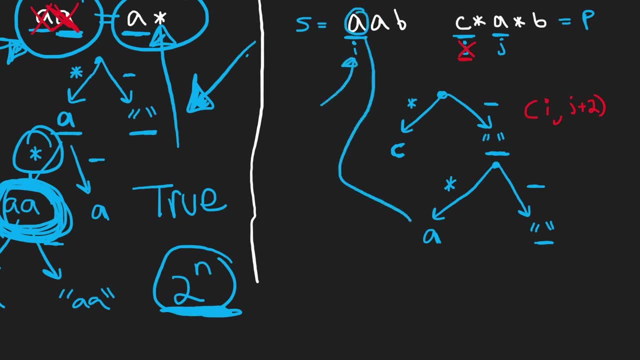 take a look at I. We matched A- exactly what we wanted to do, Right? So what are we going to do with I? Well, we're allowed to shift it by one now, So we're going to take I and move it over here. Right, We already matched this character. We don't really. 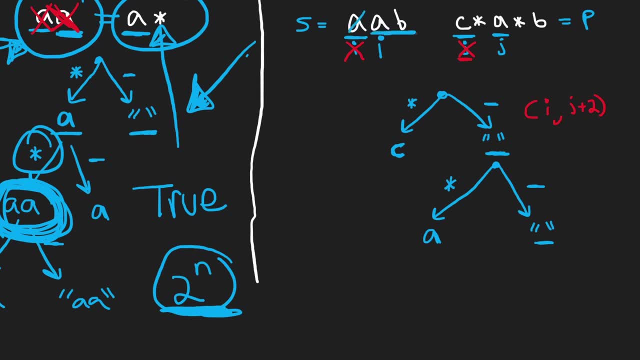 need to match it again, but we do need to match the remaining string of S, A and B. What about J? Well, J can stay the same, because we used the star once. We repeated this A once. Now we can continue to repeat it, or we can repeat it zero times, And we can make that decision by by. 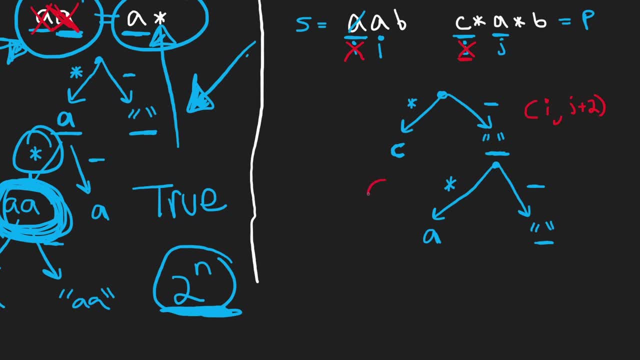 leaving J exactly where it is. So, when we go down this path, when we actually use the star, what we're going to do is add one to I, but leave J exactly as it is, And this is important too. These two things are important because this is exactly what I'm going to do when I write the. 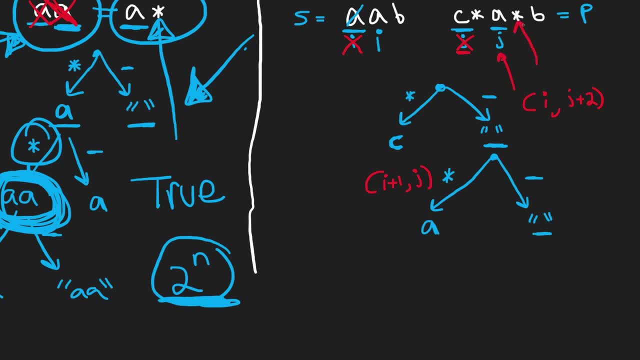 code. So since we're still at J and there still is a star that comes after it, we again have two choices. So we can choose again to repeat this A or we can choose to not repeat the A. So if we repeat the A, then we're going to have to repeat the A. So if we repeat the A, then we're going to. 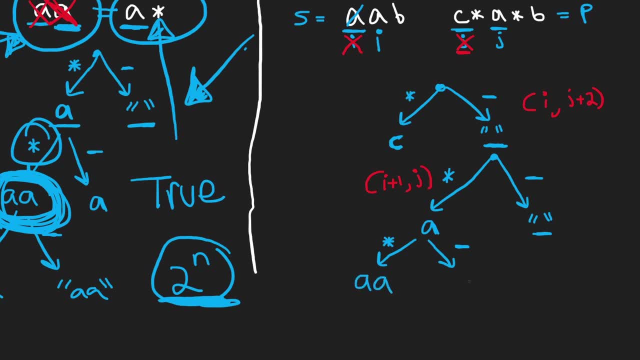 get the string double A, right, And if we choose not to repeat A, then we're going to have a single A, and then meaning we're not going to use this anymore, And then we're going to have a B that comes after it. right, And you can tell A B by itself does not match the entire input string. 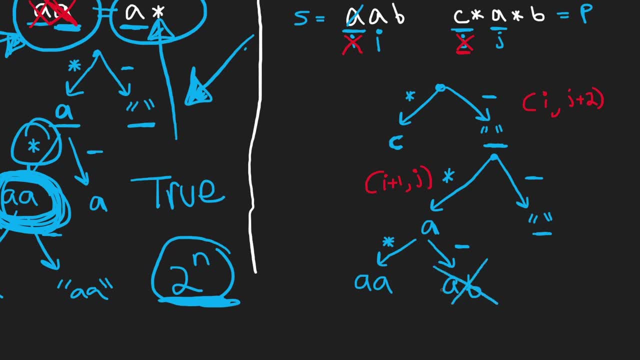 right. So clearly this is not going to be the solution, But you can see that the new character we just added, the single A. it matches exactly what we were looking for. Another A right. So that means we can repeat what we just did up here. We can take this I and shift it by one. 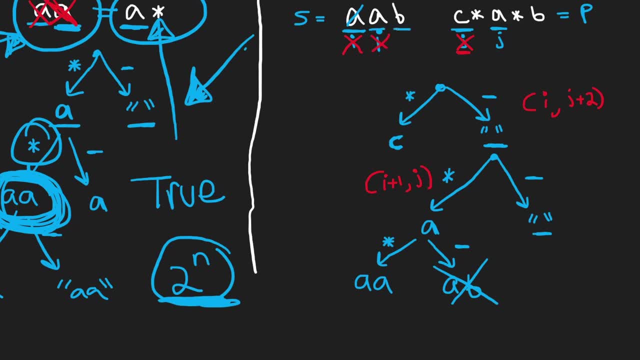 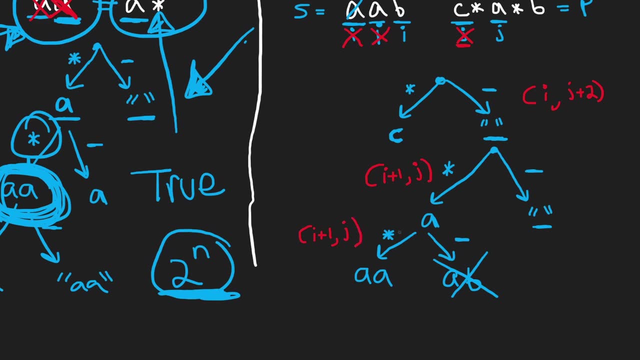 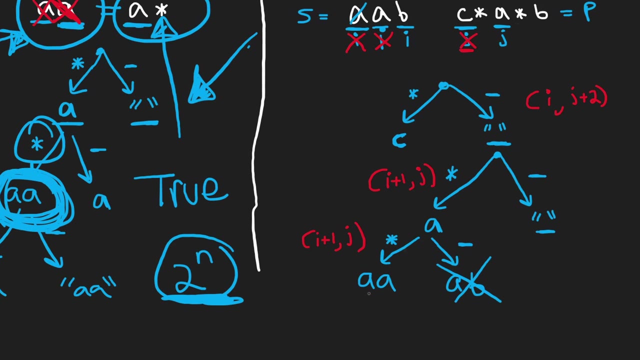 and we can leave J exactly where it is. So now I is at the last character in S and I was shifted by one and J remained the same. Okay, I'm starting to run out of space, but let's see if we can finish this Again. we're at this position where a star comes after right. J is over there, So we. 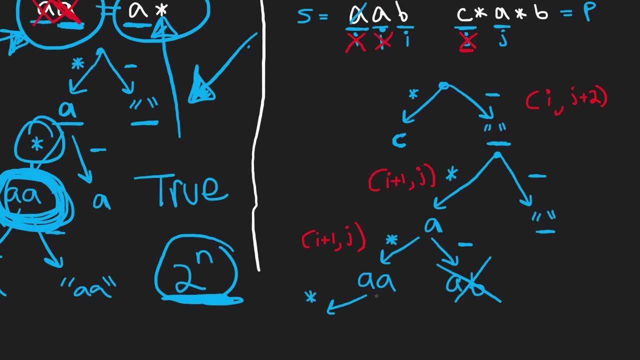 have two choices: We can use the star or we can not use the star. So we can use the star or we can use the star. If we use the star, we're going to get triple A right And see the third A it does. 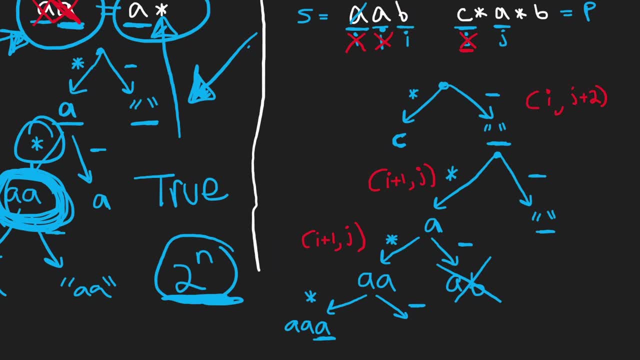 not match the character that we're currently at B. So clearly this is not going to be the decision we go down. If we don't match the A, then we're going to end up with a double A right- Exactly what we had before right, But in this case, as we usually do when we don't use the star, 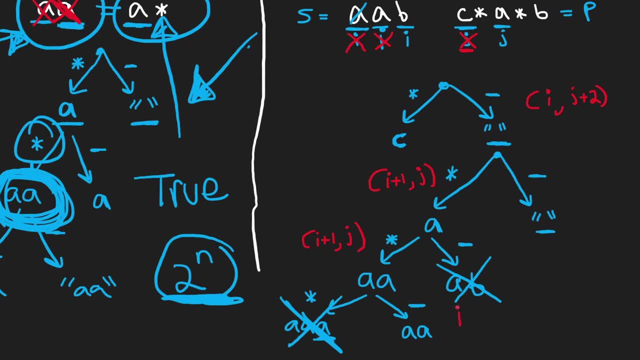 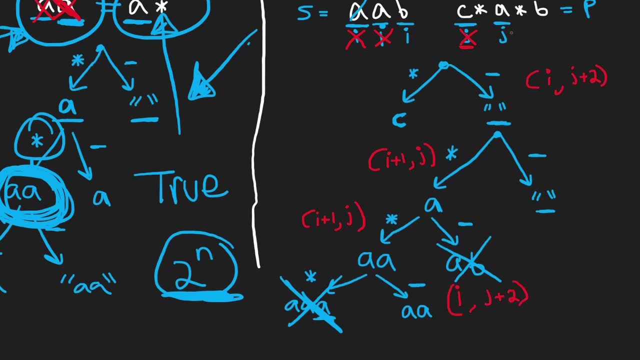 what we're going to end up doing is taking I leaving it where it is, because we know we didn't match this character right now. but we're going to take J and add two to it, And since we add two to J, that means we have. 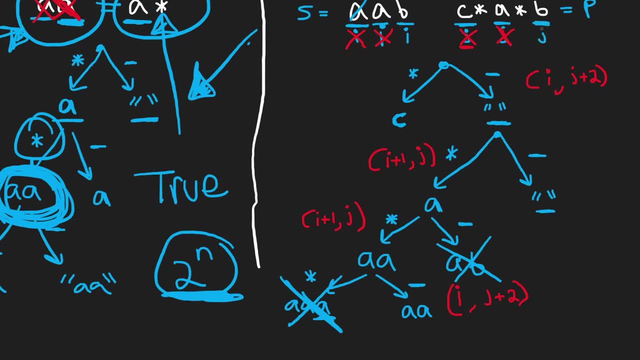 to shift it by two. So now J is going to be at the last character in P at the B, And notice how J, now the character after there's no star that comes after it, right. So we actually don't have a choice right now, We are only checking: does the character at J this B? 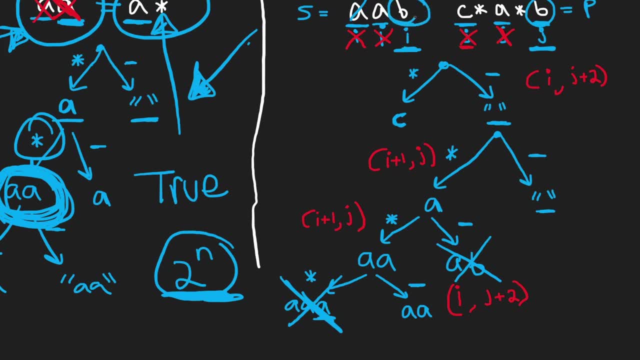 does it match the character at I, this other B. We don't have a choice, because there's no star. We're not allowed to repeat this B zero times, or one time, or three times. We have to use it only a single time. right, We must use it. We're required to use this B, but lucky for us. 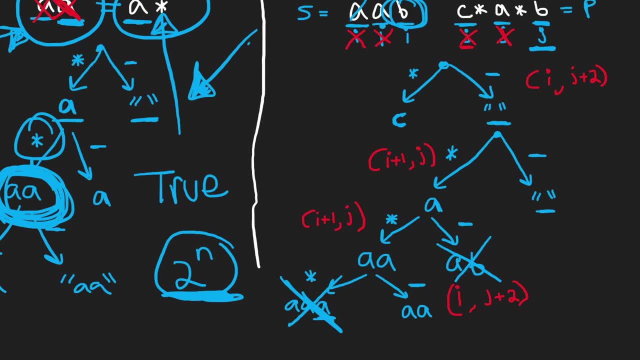 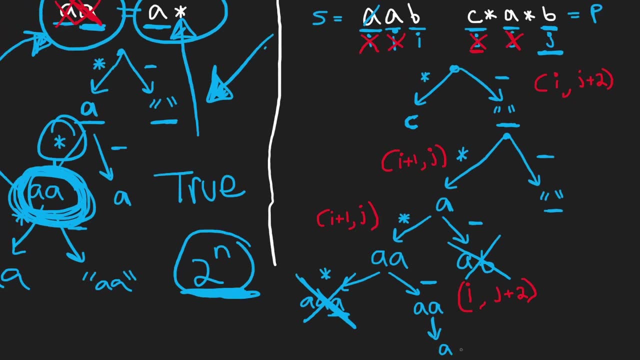 we have a B right here, right? So we don't have a choice right now. We're just checking: do they match, And they do. So what we're going to do now is see that our string that we created with our regular expression is now A, A and B right, And that 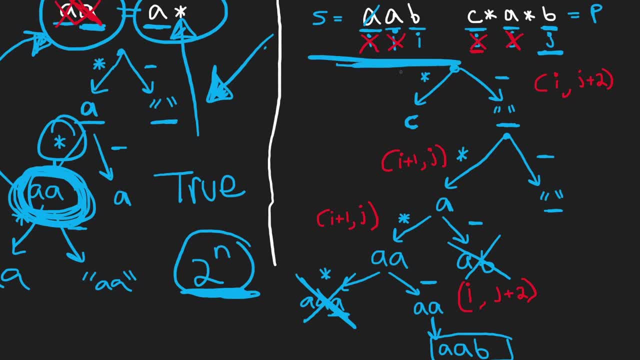 matches what we wanted to in the input string. But it's important to note when we do not have a star, we're strictly checking: do the characters equal? We're checking: does S of I equal P of J? And if they do equal, what we're going to do? how are we going to update our pointers I and J? 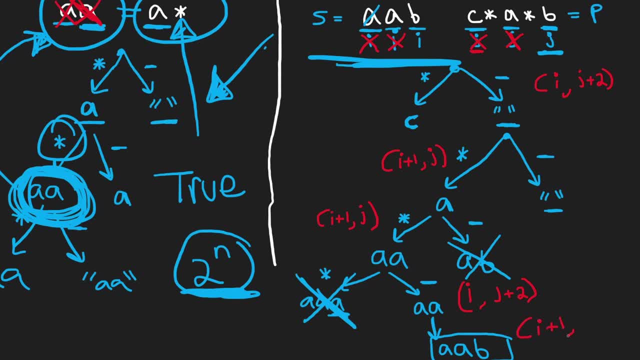 We're going to take I, add one to it, and take J, add one to it. We're going to do this in the code. So now, when you see if we take our I and then shift it over here. so I'm just going to 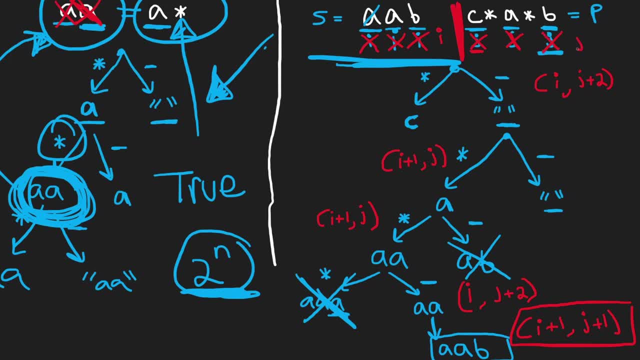 make a barrier between these two. And if we take our J and shift it by one, you see both of these are out of bounds. right, I is out of bounds and J is out of bounds. That's how you know. we have perfectly matched. So if we take our I and then shift it over here, we're going to have a barrier. 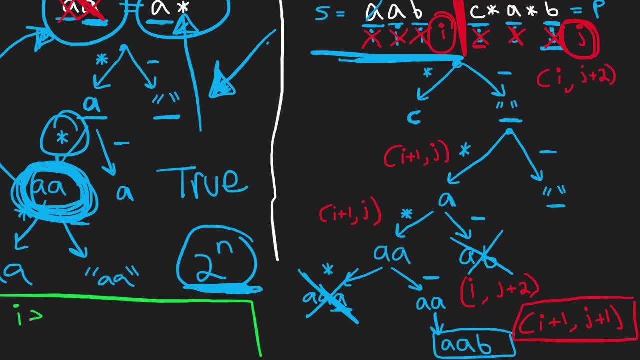 between these two. So really, when we say that I is greater than or equal to the length of S, meaning it's out of bounds, and J is greater than or equal to the length of P. that's how you know. they have matched exactly, perfectly. But my question is: what if I wasn't? was I was still? 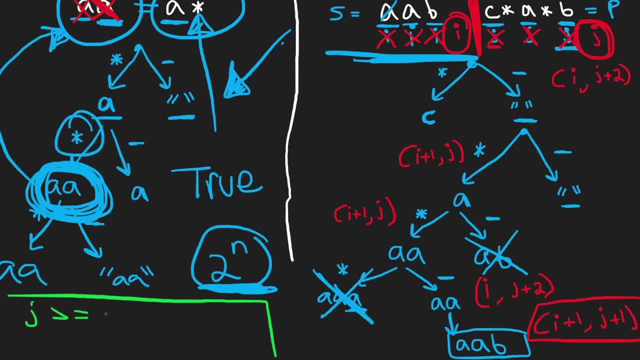 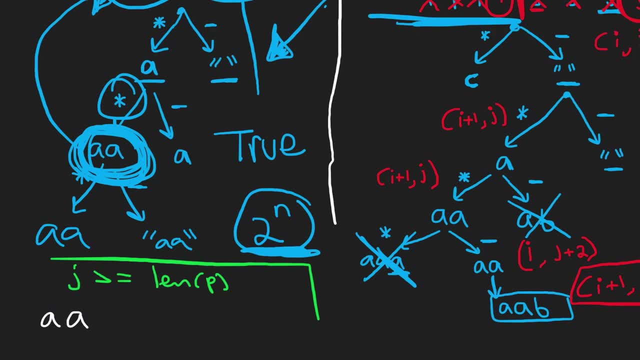 inbounds. But what if J was out of bounds? What if J was greater than or equal to the length of P? So if we take our I and shift it over here, we're going to have a barrier between these two. example would be this: let's say our input string was a, a right. that's our input string, our pattern. 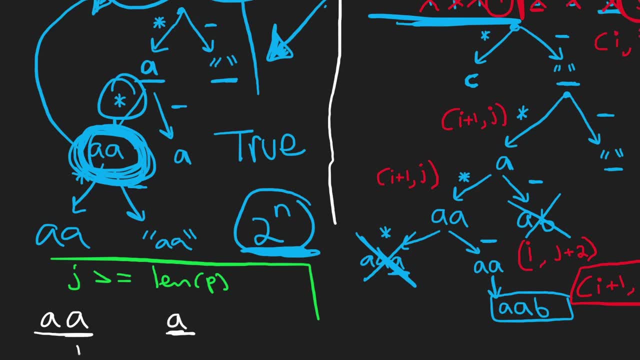 is a is just a single, a right. let's say our, our index of i was here. let's say our index of j was over here, right, clearly this does not match. this is our string s, this is our pattern p. this does not match this right. so basically, if only j is out of bounds, then they do not match. 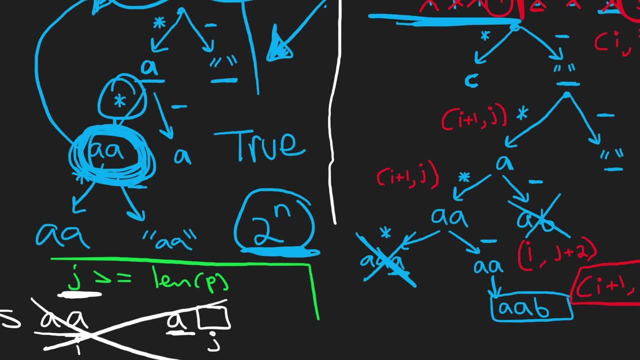 because we still have some string in the input that hasn't been matched. but what if the opposite was true? what if i was out of bounds? right, i is out of bounds, so i is greater than the length of s, but j was still in bounds. what does that look like? an example would be this: let's say we had 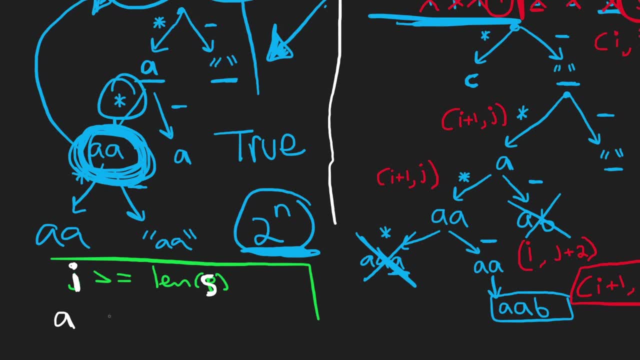 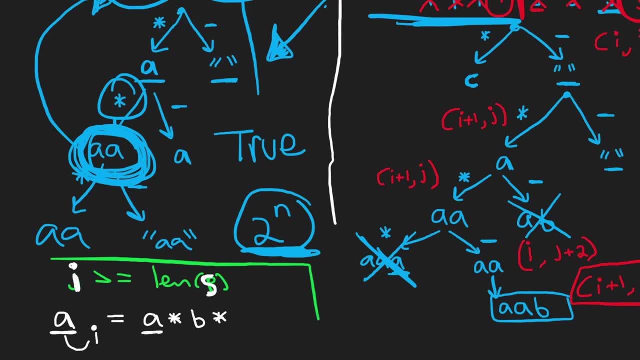 was shifted by one, so our i is over here and we took our j was shifted by one, so our i is over here and we took our j was shifted by one, so our i is over here and we took our j. starting over here, we matched the a. 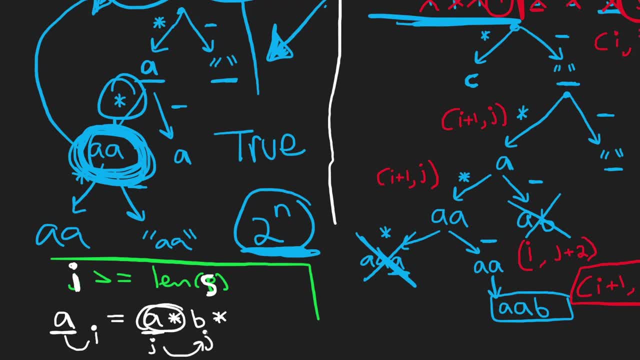 starting over here, we matched the a. starting over here, we matched the a a single time, then we shifted our j a single time, then we shifted our j a single time, then we shifted our j to be at this b character. so basically, to be at this b character, so basically. 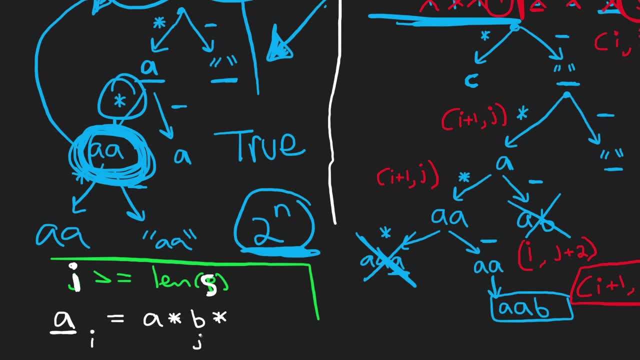 to be at this b character. so, basically, i'm asking so with our i over here, and i'm asking so with our i over here, and i'm asking so with our i over here and our j over here. do these two strings? our j over here, do these two strings? 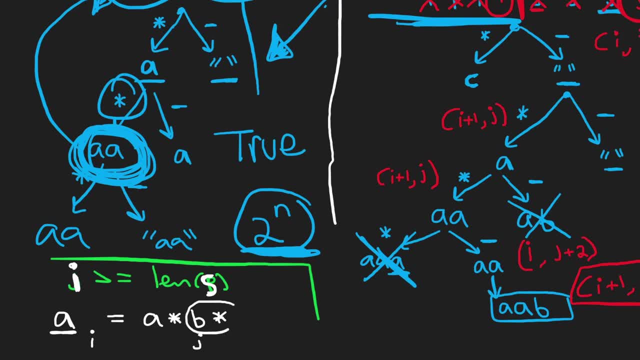 match each other technically. yes, right, because this b could be repeated zero times and still match the input a. so just because i is out of bounds doesn't mean we have to return false. but, as i just showed a second ago, if the j happens to be out of bounds, so if the j is out of bounds. 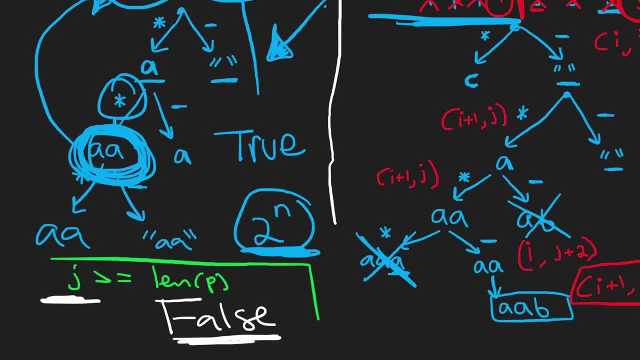 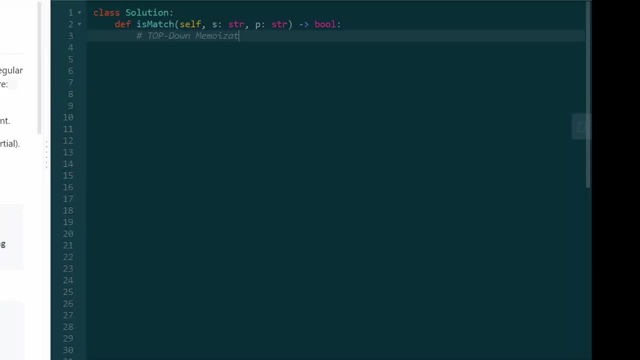 then we must return false. i know this is probably a little confusing with these edge cases, but i hope the examples make it clearer and i hope the code that i'm about to show you makes it even more clear. so again, i'm going to do the top down memoization dynamic programming solution, not 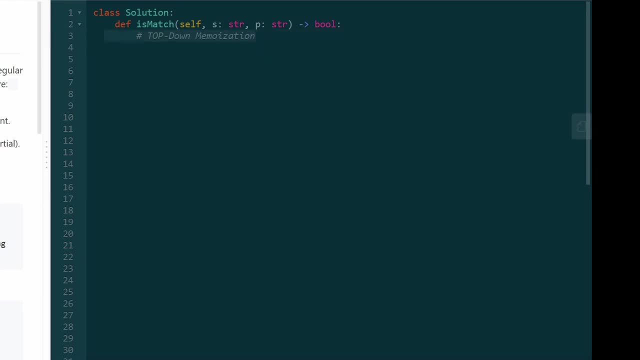 the bottom up. i think the top down is easier to understand when you're first starting this problem. just doing the bottom up solution is more confusing in my opinion. but we are going to do this recursively, so i'm going to do a nested function depth first search inside of our 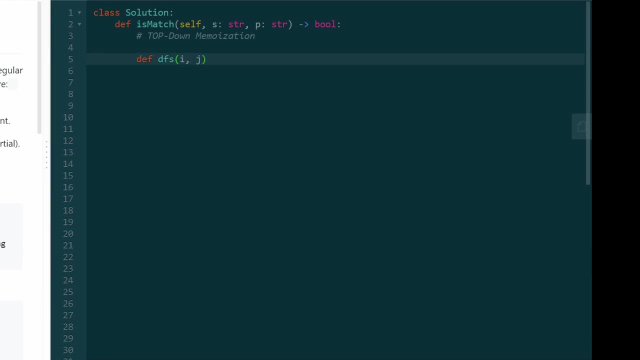 uh is match function. i guess you could call this backtracking or you could call it uh, whatever else you wanted. i'm just going to call it dfs and we're passing in i and j, which are going to tell us what position we're at in the input string s for i and j is going to tell us where we're at. 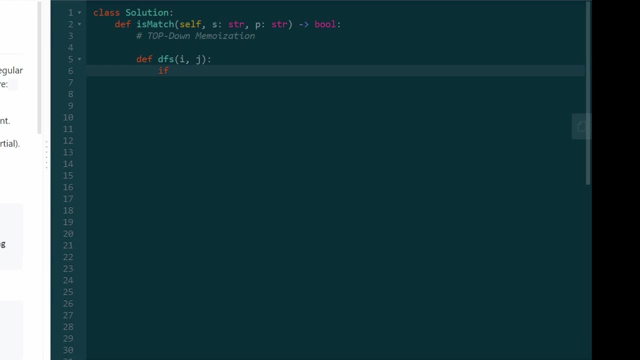 in the input string p. so, as always with recursive functions, let's start with the base case. i just showed you that if i is out of bounds and j is out of bounds, that means we have found our solution. that means we have found our solution and we have found our solution, and we have found our solution. 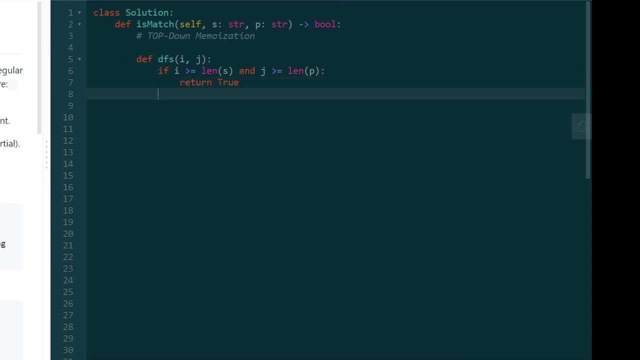 we were able to match the pattern to the string, so we can return true. but, as i showed you, if i is not out of bounds but j is out of bounds, we have some string and s that we haven't matched and there's no way we're going to be able to match it, so we have to return false. so these are our two. 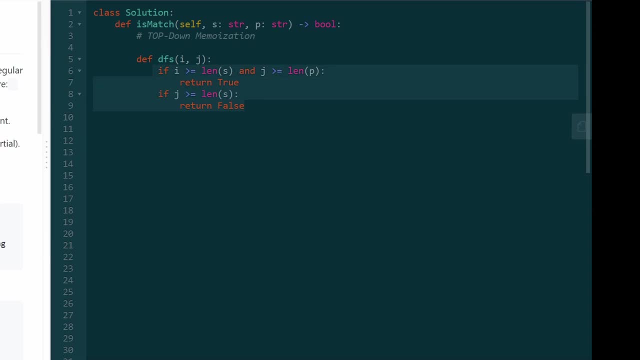 base cases. notice that, given these two cases, it's still possible that i could be out of bounds, right? i technically could be out of bounds and neither of these return statements would execute right. this needs i and j to be out of bounds, so we would pass this and we would pass this and i could. 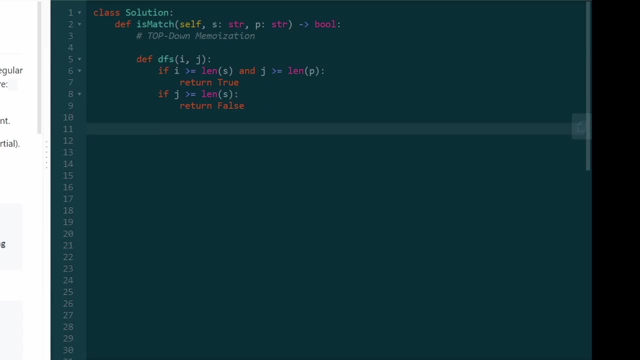 still be out of bounds, but i'm going to show you how i'm going to handle that right now. so the first thing we want to check is: is there a match between the first character, so is there a match between s of i and p of j? and the other thing we could check technically right: p of j could have a period in. 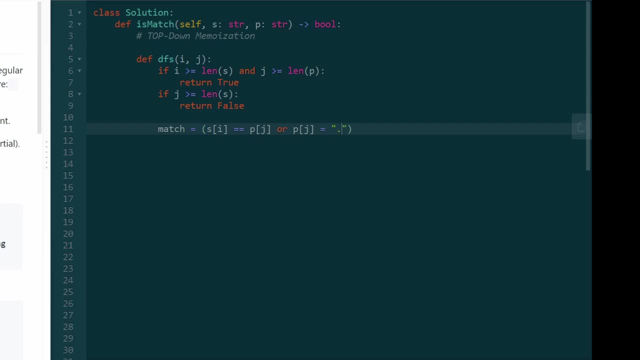 that position, meaning the period, matches the first character and the other thing we could check is to any character, right? so we have to check this or check this, and since we know i could technically be out of bounds before we even check this, we have to confirm that i is in bound, so i is. 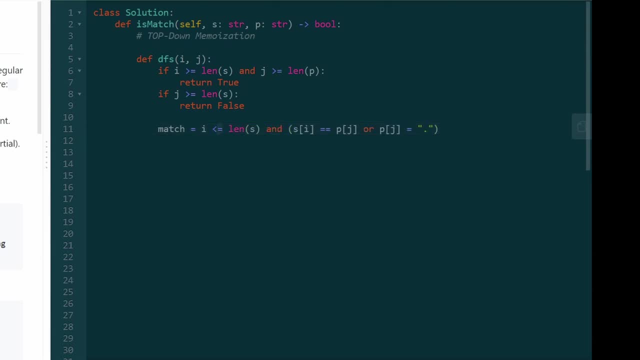 less than the length of s, so strictly less than, not less than equal. so if these conditions are satisfied, that means the first character of each string matches exactly. the reason i'm putting this in a variable is we're going to have to repeat it a couple times, so we're going to have to repeat it. 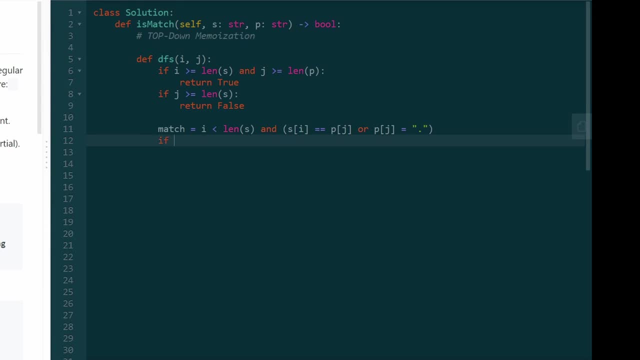 a couple times in the following code. so the first thing i want to check is: does the following character in the pattern string, so p of j plus one, does it match the star? is it a star? and the reason i'm checking this first is because the star has the highest precedence and i'm checking j plus. 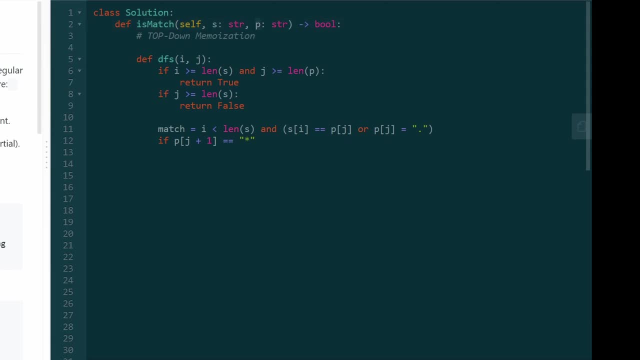 one, because we know the pattern. the first character in the pattern string is never going to be a star. and since i'm checking p of j plus one, i have to first check that j plus one is a star. and i'm checking j plus one is in bound, so i have to check that it's less than the length of p. so if 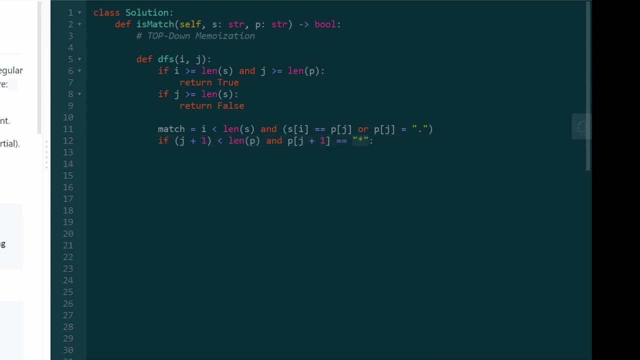 this is true. that means we're gonna have to, we're gonna have to take care of this star right, and we remember when we encounter a star, we have two choices. so i'm gonna do a recursive call right that first search. the first choice we have is: don't use the star right. if we don't use the. 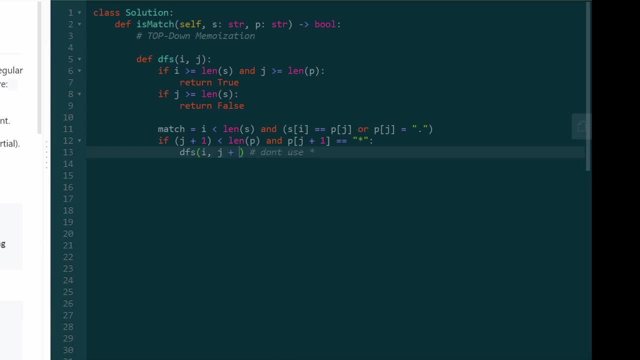 star. we leave i as it is and we take j and add two to it. right, that's one. now we know we have two choices. if either of them evaluates to true, then we can return true, right, we're brute forcing this right now. so the other decision we have is: the other decision we have is: 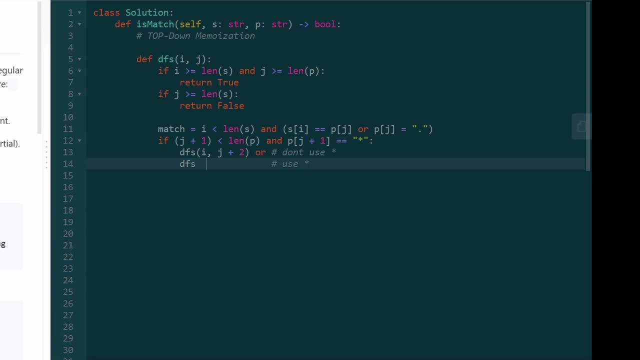 use the star right. so if we use the star, that means we can take i and add one to it and we can leave j where it is. but remember, we can only use the star if there's a match between the first character- right, the first character and the first character, and the first character and the first. 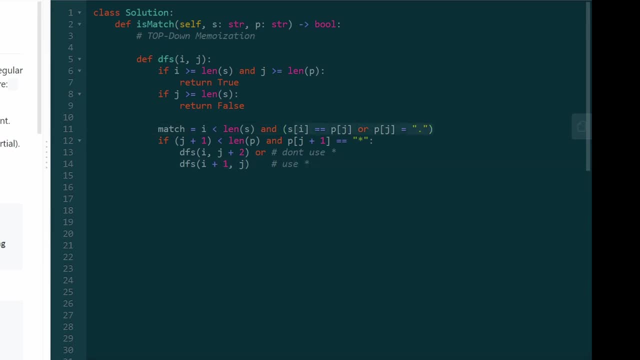 two characters right, because we only want to use the star if there happens to be a match. so really, here we're checking if there's a match and this whole thing about this recursive call evaluates to true right. so i'm going to wrap this in parentheses. so basically, what i'm saying is: 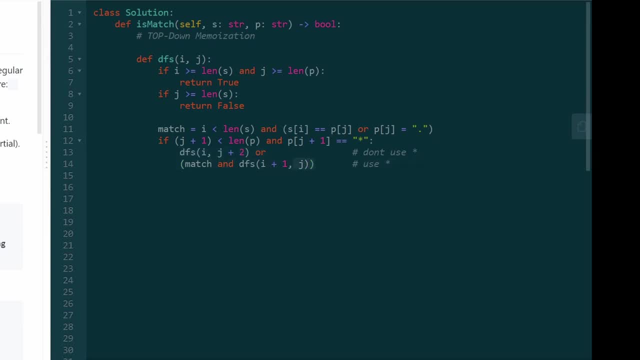 these are our two choices. this is one recursive call and this is another recursive call. if either of these evaluates to true, then we can return true, and that's what i'm doing, basically, by putting these on the same line. so i don't know the best way to format this. maybe this is somewhat readable. 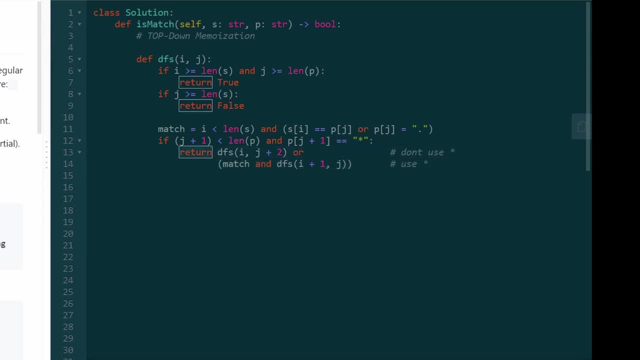 so if either of these is true, we're going to end up returning true. if neither of them is true, we're going to return false. so this by itself, this, these three lines of code, handles that star for us. now, if this isn't true, meaning we don't have a star character, then we're looking just for a simple 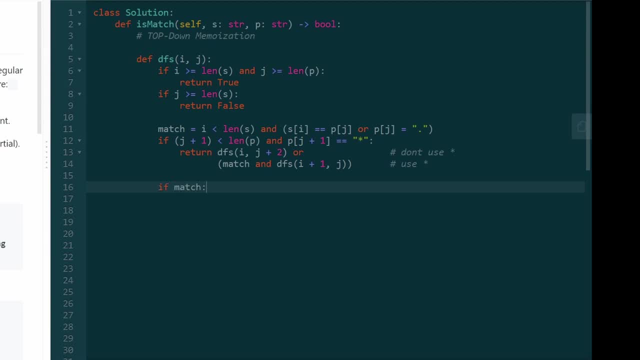 match. right, so we can just check if match. if the two characters are the same, then we're going to return false. if the two characters match, then what are we going to do? well, remember? we can then increment i by one and we can increment j by one and return the result of that. now, if there's not, 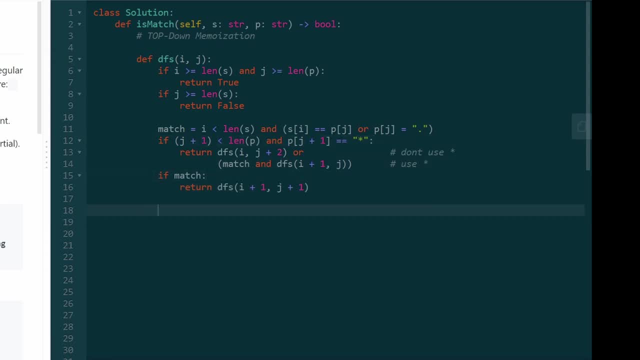 a star and the characters don't match. in that case, it's simple, right, then we can just return false, meaning that this string will never match the pattern. so then we return false, and this is the brute force solution. it's actually as simple as that. so let's, let's return it. and let me show. 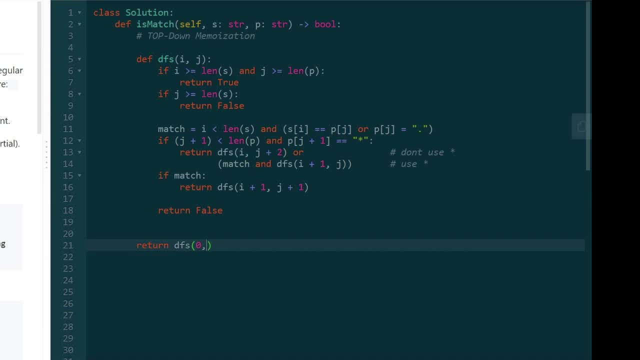 you how inefficient it is, so let's return it. and let me show you how inefficient it is. so let's return it. and let me show you how inefficient it is right now, so we can call our depth for search starting at zero in both of the strings. oops, i had a syntax error, so we had double equal over. 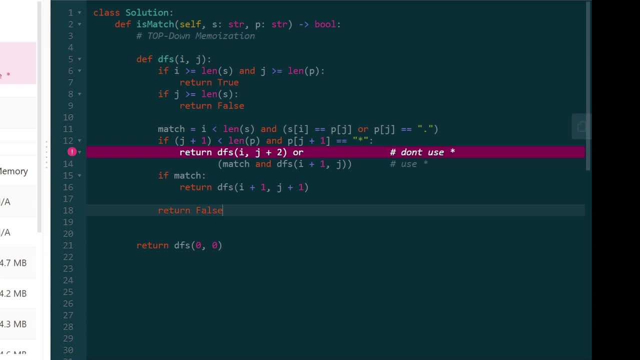 here. we have to put double equal over here, oops. and one last thing: when you have multi-line stuff in python, you have to wrap it all in parentheses. so i'm just going to wrap this entire thing in parentheses. hopefully it's still readable. and a third bug. so i don't know why. i checked if j. 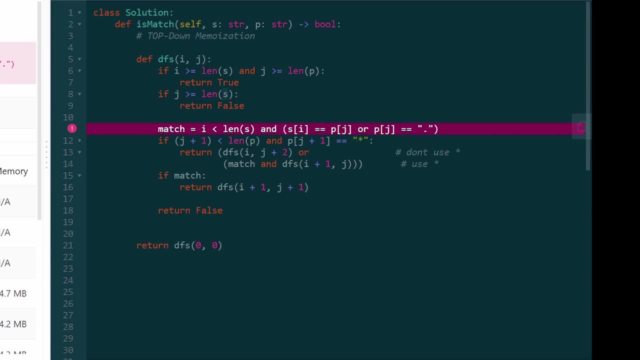 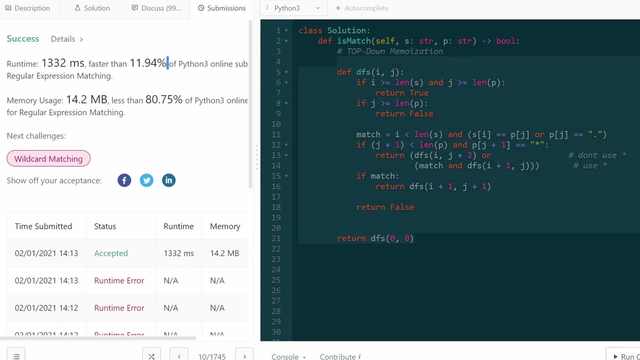 is out of bounds of string s when j refers to the index of string s, string p. so sorry about these bugs, but okay, so this time it finally worked. you can see it's not super efficient, right, it took about. i think this is 1.3 seconds and it was 11, so we did the top we. 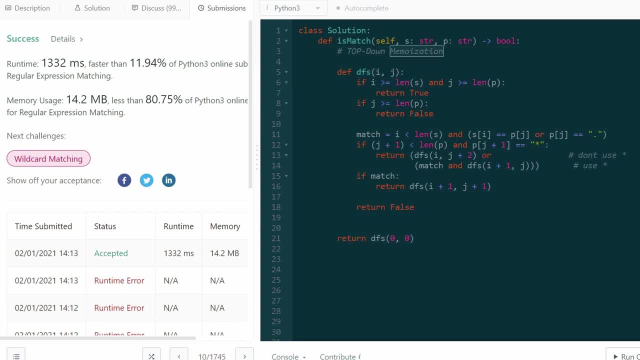 did the brute force solution, but look, i forgot to do the memoization right. so let's actually do the caching now and make this efficient. so i'm going to create a cache. it's going to be a hash map, so before we do anything, whenever we call this function, we're first going to check. 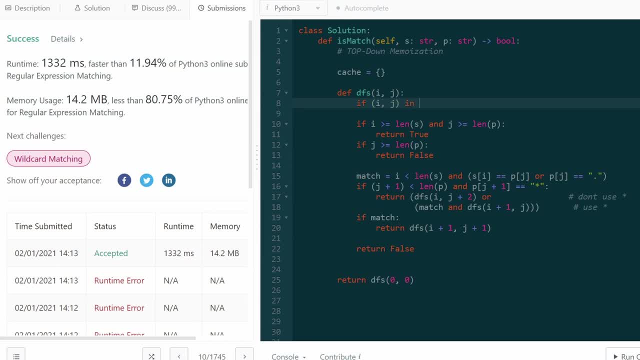 if i, if the pair i- j- has already been added to our cache. if it has, then we can return it right. so this is going to basically not have to. it's basically going to take care of repeated work for us. if we execute this, we're not going to have to do all the repeated work, but now we 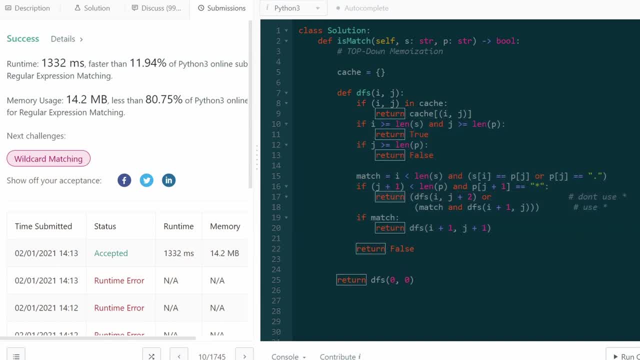 actually have to use this cache. so instead of returning this right away- you can see down here- i'm going to actually take this and add it to the cache. so at index i j i'm going to put the value of this returns to, and after that, after we add it to the cache, then i'm going to return it and i'm 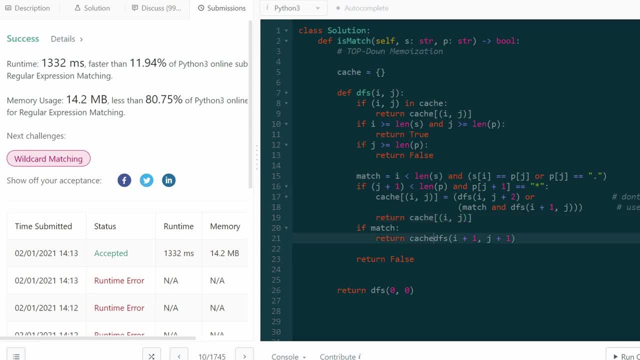 going to do the exact same thing down here, so adding this to the cache, and then we can take this and return it. so we're all we're doing right now is caching the work that we do, so we don't have to repeat it. lastly, down here we can say in the cache, add false and then return false. so basically, by 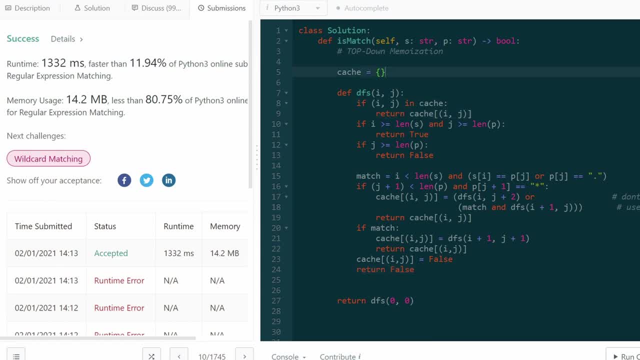 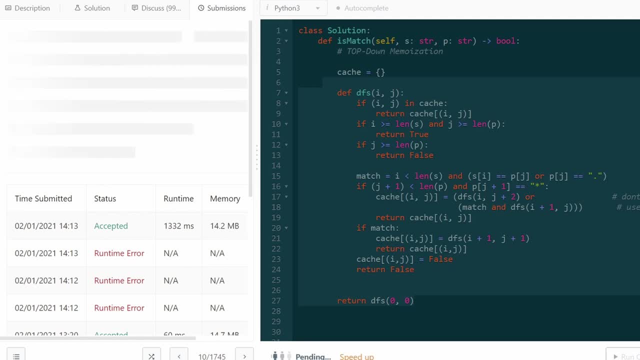 just adding what like four or five lines of code. we've added the caching element to this function. it was pretty easy, so taking the brute force to the uh optimal solution was actually pretty easy. and look at the result. look how much faster this is 44 milliseconds, 81. so we actually didn't even 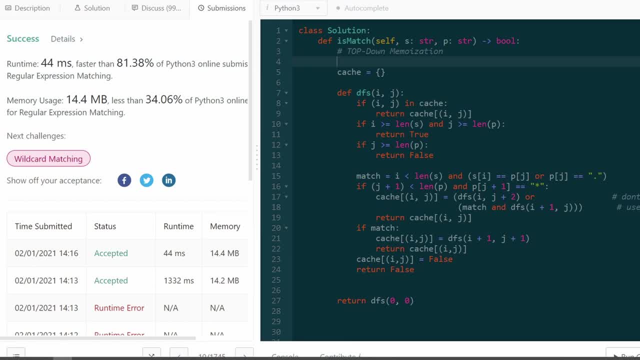 need to do the bottom-up dynamic programming solution right, and this, i will be honest with you, is not the prettiest way to write this code. i've seen solutions like this, where you have to 소위 말하면: 포함된 시스템, 적용, 수단에, 적용 프로그램에, 적용. 할 수, 없을, 수, 없죠. 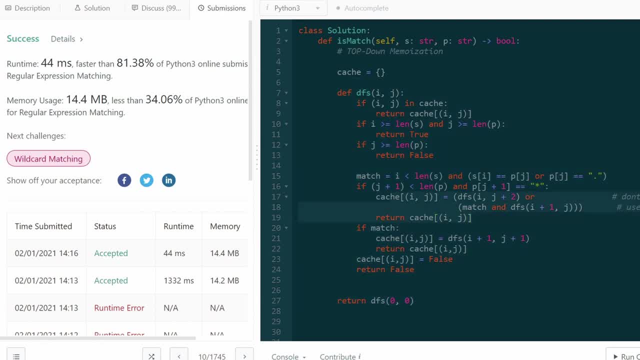 but i really hope that you were at least were able to understand what we're doing right. the, the meat of the work is done in this call right. basically, these two lines of code are the work that we're doing right. this is where we're handling the star case, and you can see it's. 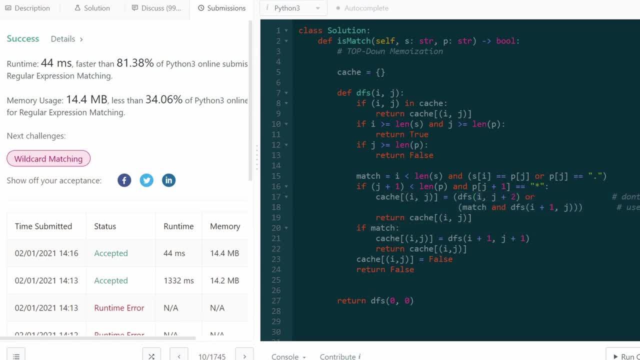 actually not that difficult, right? all we're doing is: i stays the same, j added two, or i plus one, j stays the same and that's it. that's what we want to do right now. let's see what we do. now we're going to write the next answer for our solution, right? let's take a look at the previous example here.